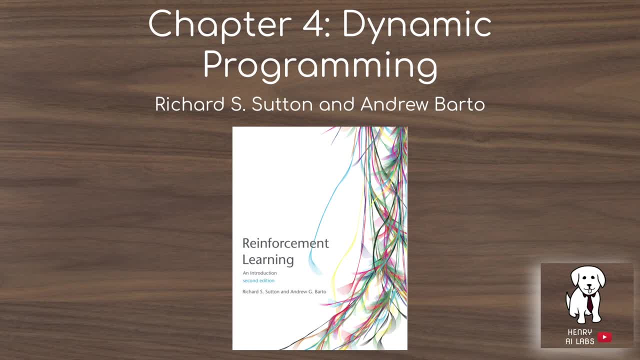 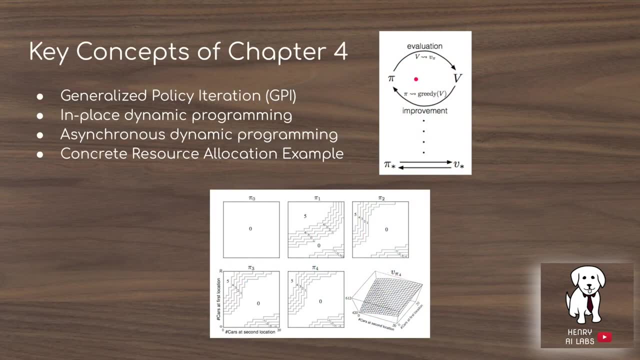 ideas. A free PDF version of this book is linked in the description, as well as a print version if you want to buy it. Although Chapter 4 is titled Dynamic Programming, the key takeaway is pictured here: generalized policy iteration. Compared to Chapter 3, where we use Bellman Optimality. 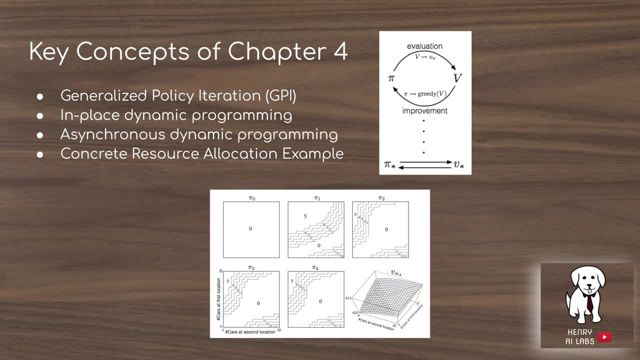 Equations to derive a system of equations to solve for the optimal value functions. the generalized policy iteration is a technique of iteratively approximating and getting closer and closer to the optimal value functions, And this is much more computationally tractable, especially when you have large state spaces. So we'll also talk about components of Dynamic. 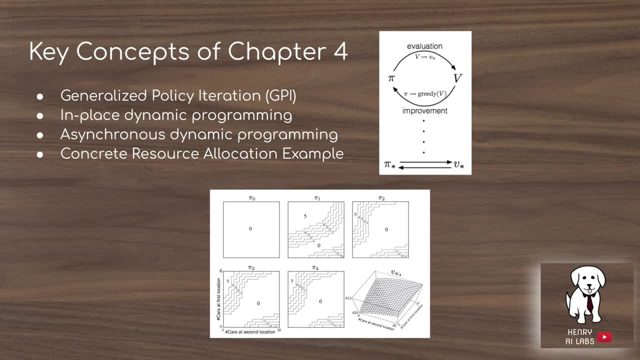 Programming like in-place Dynamic Programming to save you memory in your value function state table, and then asynchronous Dynamic Programming where we update just a subset of the state space compared to doing an entire state space sweep of the value functions, which is a very important part of the dynamic programming. 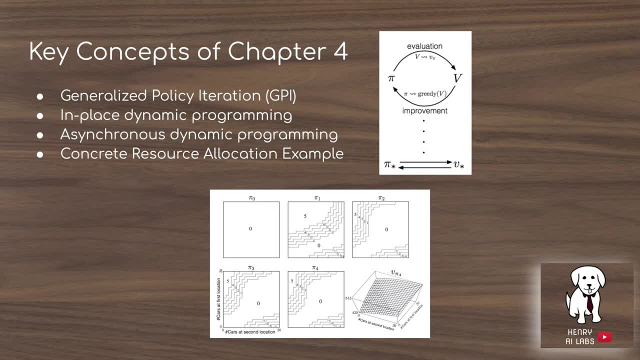 So we'll talk about that in a little bit, And then we'll talk about the dynamic programming, which is totally impossible for things like backgammon with 10 to the 20 states or chess or many of these other reinforcement learning problems we're interested in Throughout the 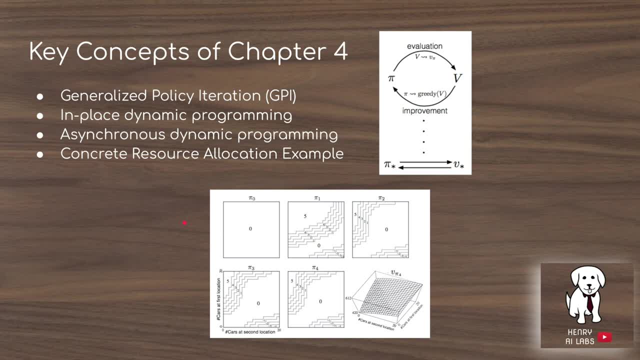 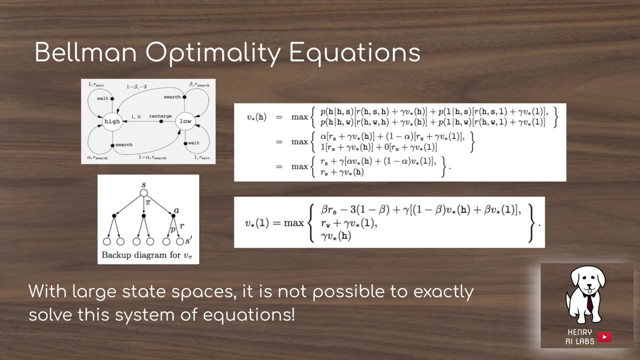 chapter. we'll motivate these examples with a concrete resource allocation example. imagining that we have a car rental business and we are making decisions or actions to move cars between different locations, And the number of cars at each rental location represents the states of the environment. Before we get into the generalized policy iteration, let's 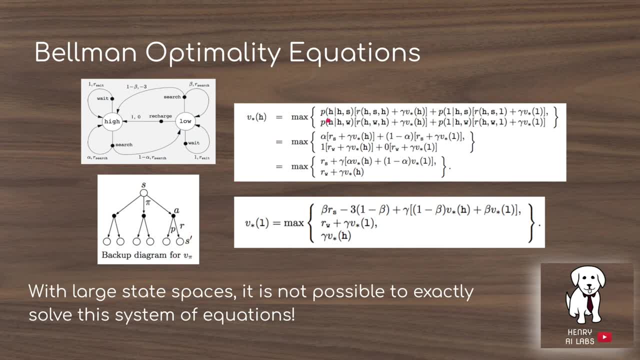 take a look at the previous chapter, chapter three. So what we did in this case is we used the Bellman optimality equations to look ahead to the future states and then use the reward that we achieve at the current state and then add it to the discount factor times, the 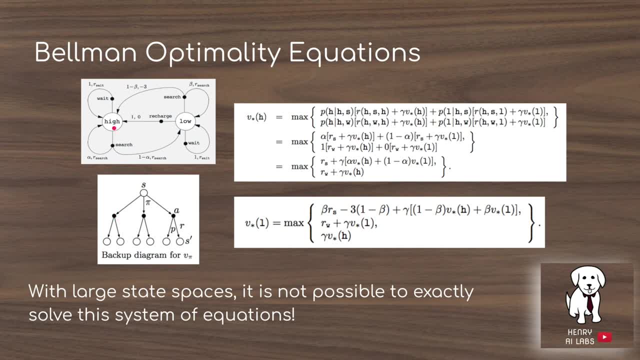 expectation of the next states that we can achieve So from high. we have the option of either searching and receiving this reward for searching, and then we have the discount factor times, the value estimate of the next state as well as if we wait and return to. 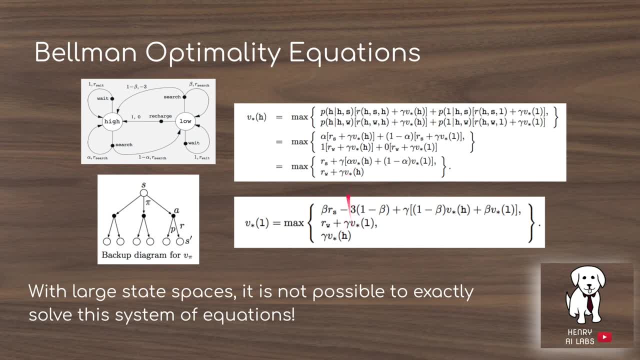 the state as well. So in this case we're able to derive the system of equations which we can solve relatively easily because we only have two states and a maximum of three actions at the low state. But when we have large state spaces, like in our car rental allocation problem or 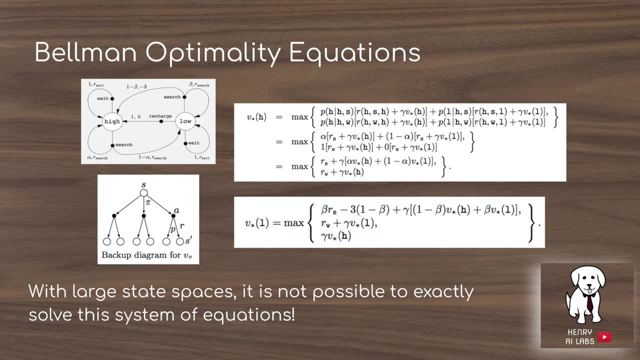 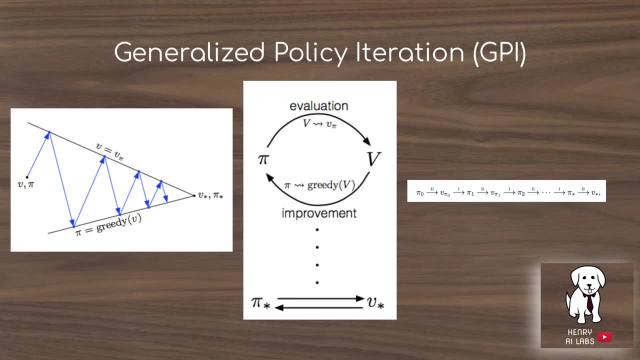 chess or backgammon or many, many of these reinforcement learning problems. it's really not possible to solve this system of equations explicitly Generalized policy iteration is an iterative approximation algorithm which is one of the most popular classes of algorithms in computer science and machine learning. So the way that this algorithm works is we randomly 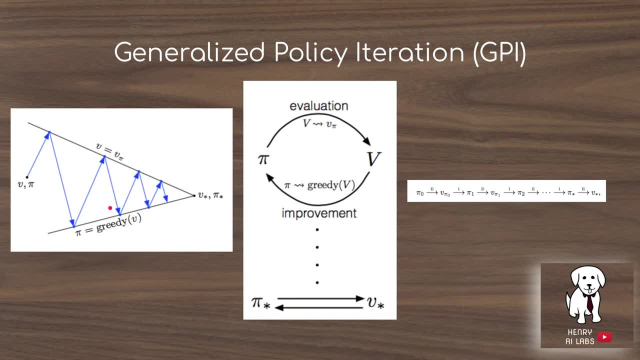 initialize our value function estimates of every state and start with a random policy. Then we proceed by evaluating the values of every state with respect to this random policy and then we update our policy by making greedy action choices with respect to the value functions of this policy. So the way that the greedy action selection works is basically you. 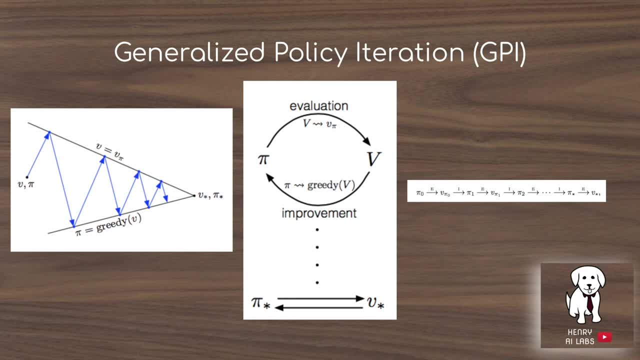 just choose the action which takes you to the state that has the highest value estimate for that state. So, overall, this generalized policy iteration algorithm loops itself until it converges to the optimal value function and the optimal policy, And this leads to a sequence of 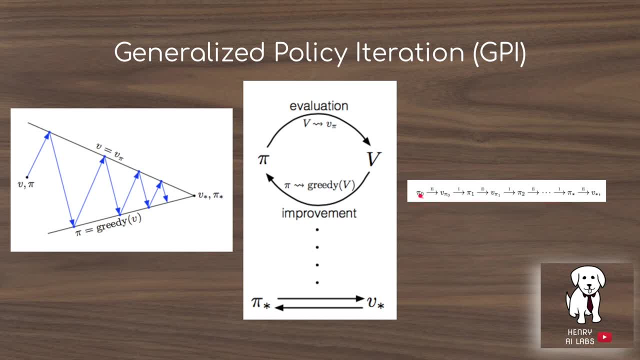 policies and then value estimates with respect to the state, And then we go back to our policy with respect to that policy, such as this: having an evaluation of the policy, then an improvement of the policy with respect to the value estimate and then evaluate improvement until it. 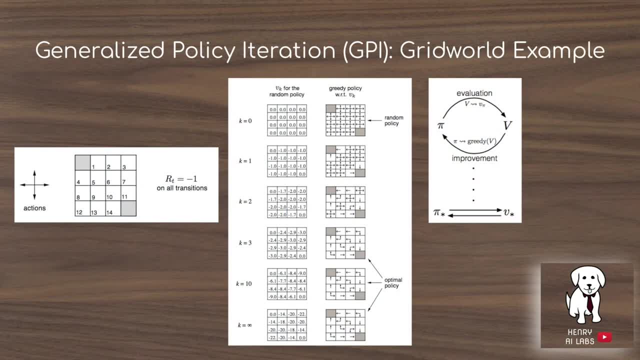 converges to the optimal policy and value function. The generalized policy iteration algorithm is probably best understood with a concrete grid world example. So in this case we have this grid world where we receive a minus one reward for every state, except for these gray shaded boxes. 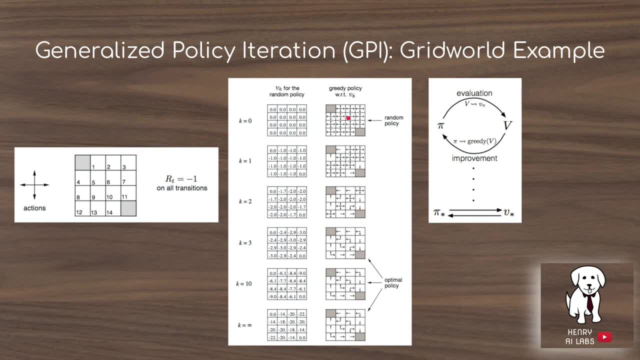 which is where we receive zero reward. So we initialize our policy to be making random up, right, down, left decisions, all with the same probability. And then we initialize our policy to initialize our value estimates by placing minus one everywhere, but zero on the terminal states. So 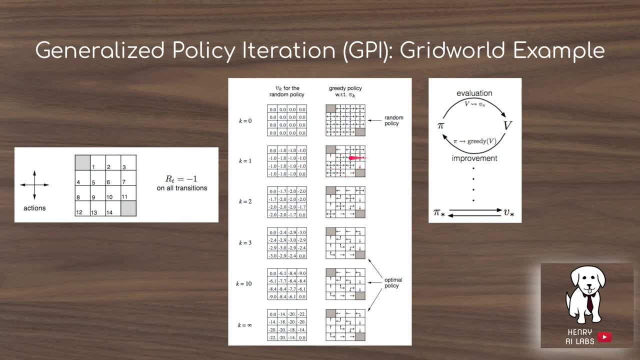 already. we have this value function here And we can see here how we make the policy greedy with respect to the value function estimates. So see how in this state, we make the decision to move left because we're moving from this minus one state. we can either move to another minus one. 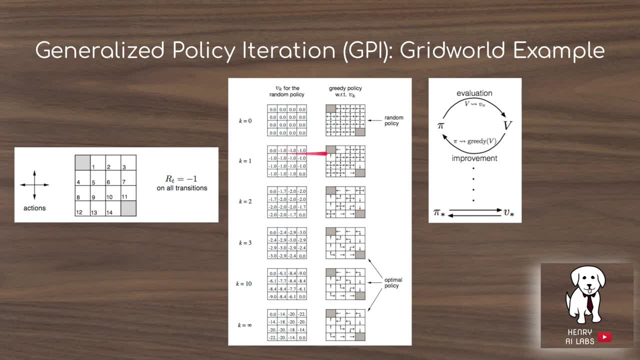 state. this right is minus one state, or we can go left, which is the zero state. So this is what it means: to make the policy greedy with respect to the current value estimates of the states. So now that we have this new policy, 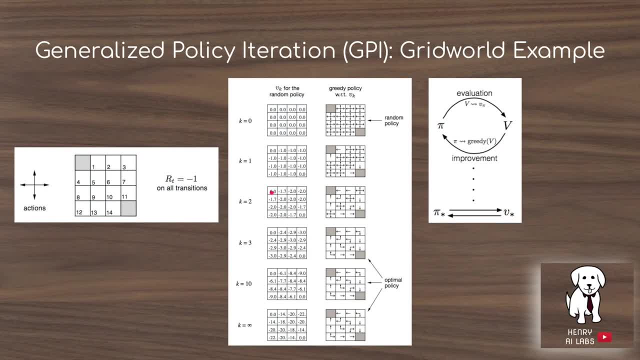 this state is is leading you into a zero reward. we can now estimate it with the Bellman equations, which leads us to being minus 1.7, rather than the minus two of its neighbors, And we repeat this until we reach the optimal policy and the optimal way of moving towards one of these shaded boxes. 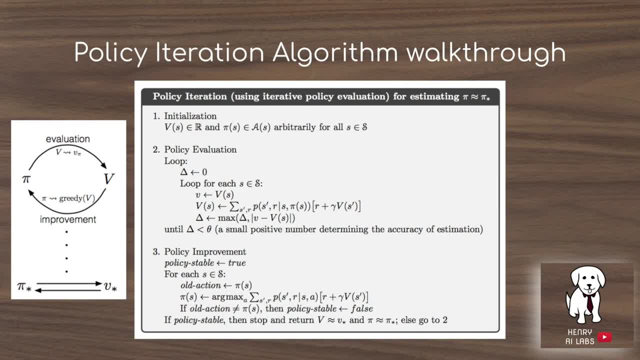 given whichever state you're currently in. Now that we've seen the grid world example, let's formally walk through the pseudocode of the generalized policy iteration algorithm. So we initially initialize our value estimates of every state, and then we have some random policy, and then we loop through this, evaluating the policy, and then 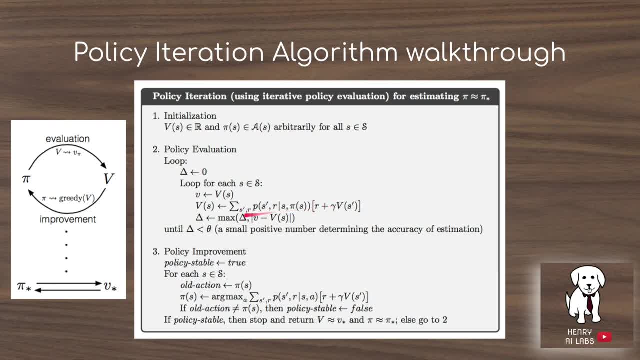 improving the policy. So the way that we evaluate the policy is with our Bellman equation lookup, where we have the MDP dynamics of the transition probabilities and the rewards, And then we use the discount factory times, the estimate of the next state that we're leading to with the action. 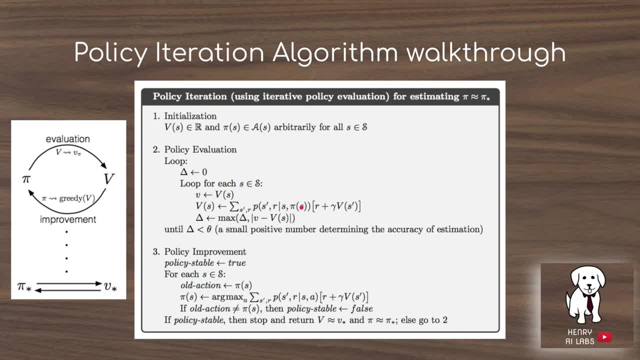 that we're taking with, then the policy, the policy parameterize by S here is giving you the action that the policy is making you take, is mapping you from the state to this action: pi parameterized by s. So then what we do is we have this delta to stop our policy evaluation. 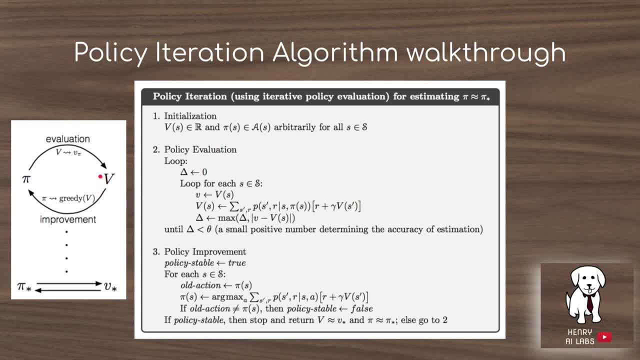 because we see here that there's an inner loop within our policy evaluation. So even in here we're looping through the v of s to make it converge to some value function estimates of the states, given our current policy. So if this delta, meaning that the update to the value of 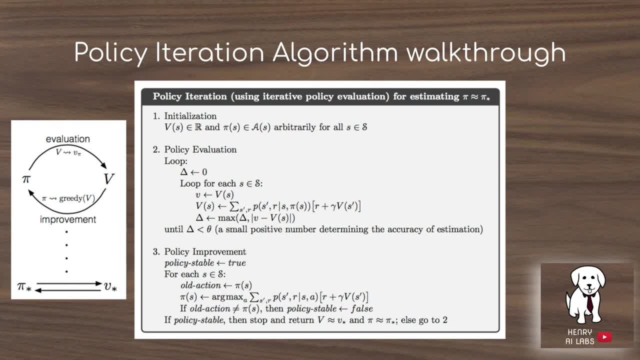 each state isn't that large, then we decide that we've successfully evaluated the policy, and then we return now to improving the policy by making it greedy, And the way that we make it greedy is by using this argmax, a meaning that select the action which takes you to the s prime state that has the 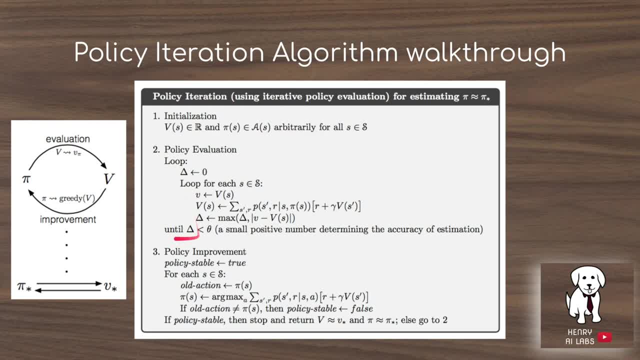 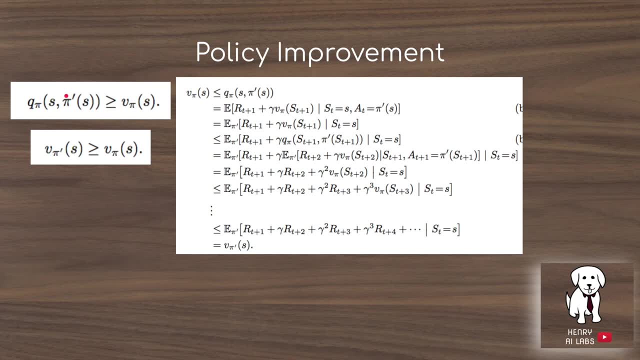 highest reward with respect to the value function estimates that were just made in step two. When we're improving the policy, we're selecting the action that is going to take us to the next state with the highest value estimate, according to the value function estimate that we just did in step. 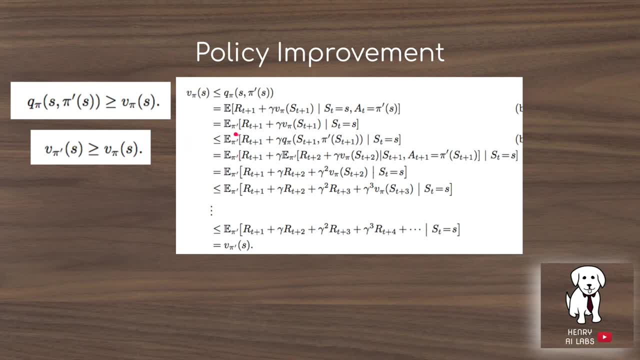 two of the generalized policy improvement algorithm. So this proof and this derivation is showing that if you update your policy to pi prime for this current state, then it's going to be better than the original policy- pi for all states- because it is the same policy in every other way and taking this greedy decision is always going. 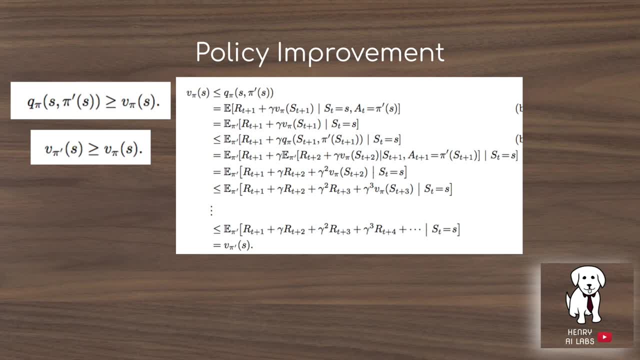 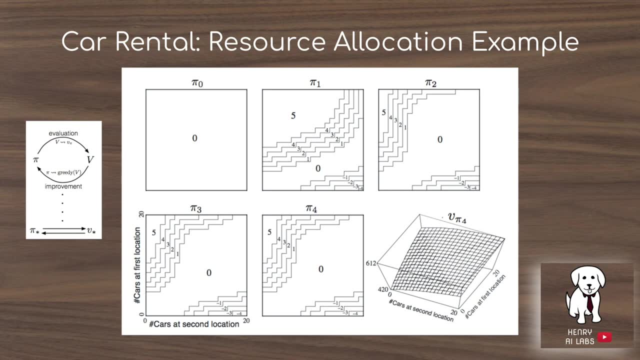 to make it better and not worse, and this is an important property of the convergence of the GPI algorithm. Next, we'll motivate our dynamic programming and our generalized policy iteration in the context of assigning resources and the car rental problem. So the states in this example: 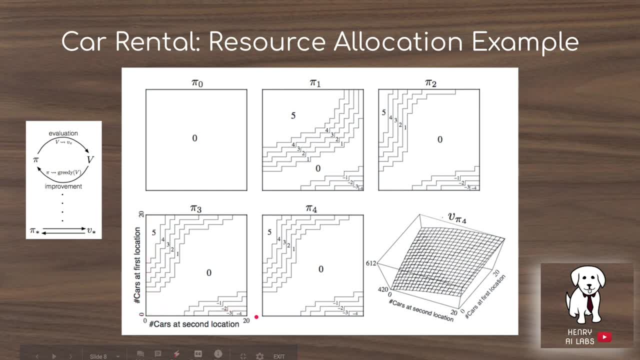 represent the number of cars at each of the locations and the number of cars at each of the locations. So if we're going to do a car rental problem, then the actions are these decisions to move cars from location A to location B, and then there's some 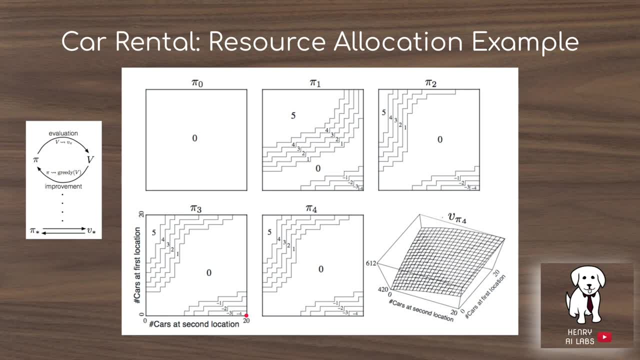 random variables in the environment that determine things like whether the cars are returned to the location at the end of the rental and then what the demand of the customers is for cars at each say time interval like a day. So this progression shows how the policy is improving in the GPI. 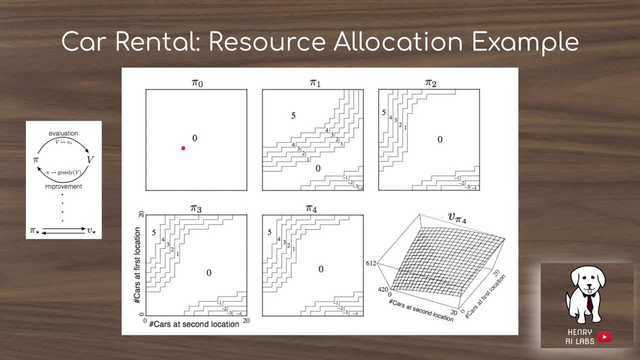 So originally the policy is just making random decisions, the zero denoting that it doesn't move cars from location to location at all. and then it starts to evaluate the values of you know which distribution of cars at location A and location B you have. So you can see in the converged policy. 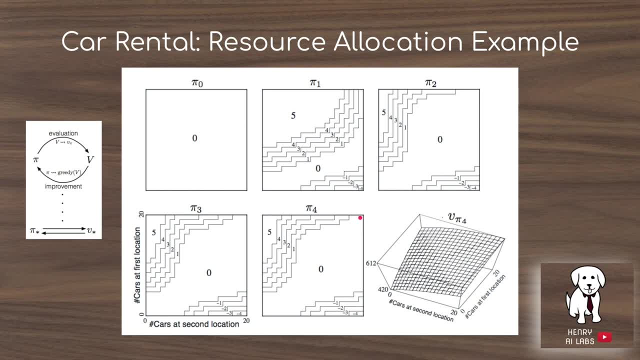 in the case when you have 20 cars in each location. this is optimal and you don't move any cars anywhere. But if you're in this case, where you have 20 cars in the first location and then zero at the second, you would move five from the first to the second, which you know. it only makes sense. 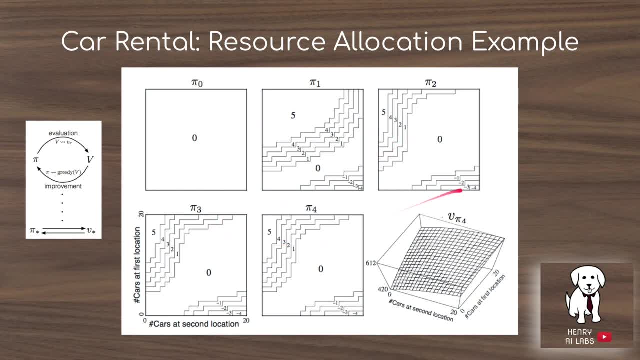 So we see this progression of the policy and I think that's the most important thing to take away from visualizing this example is seeing how this iterative policy evaluation algorithm leads to this convergent policy on the resource allocation problem. So one of the interesting characteristics 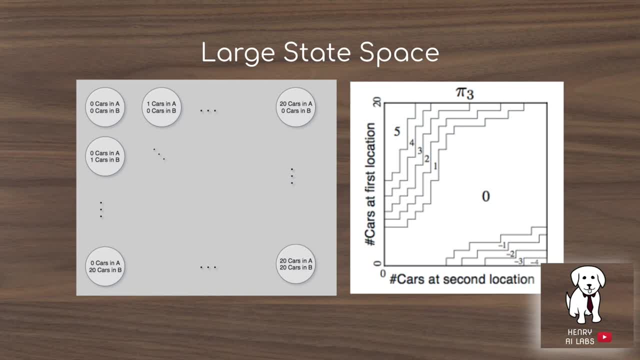 of this car rental problem, compared to the recycling robot MDP that we've seen in the previous chapter, is that we have a large state space. We can either have zero cars in A, zero cars in B, all the way up to 20 cars in A and 20 cars in B, And then we have this contour map. 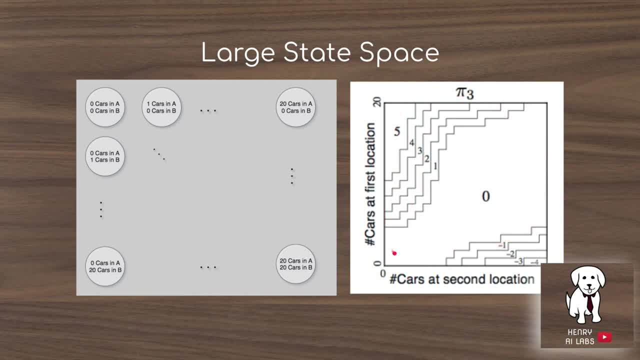 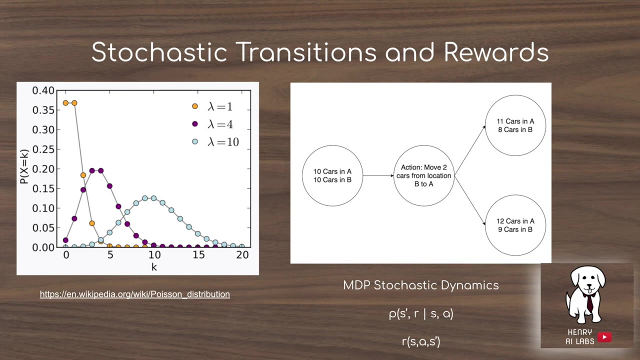 depicting our policy decisions sort of like granularizing each of these steps is would be a very like tedious diagram. So rather we have this contour map that shows a particular policy for different states. Another interesting detail of the car rental MDP problem and the example that we're using for resource allocation is that we have a different method. 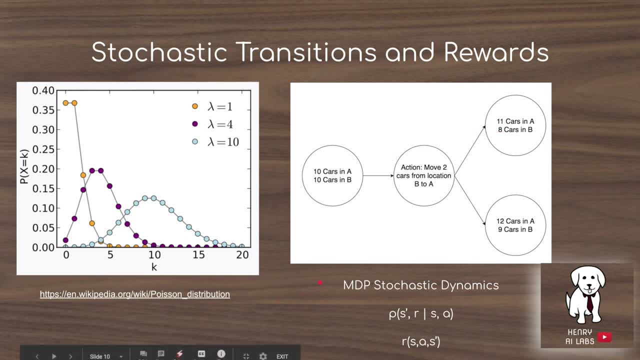 of stochastic transitions and rewards. So we saw in the recycling robot how we have the alpha and then one minus alpha and the beta- one minus beta- of transitioning from state to state given a certain action. But in this case, not only do we have this stochastic transition, it's parameterized. 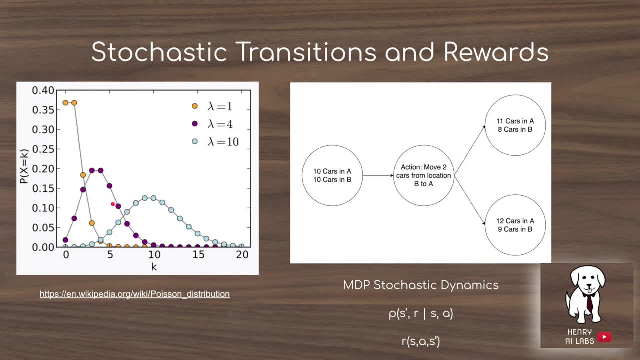 in a more complex way. So the way that the returns of the cars and then the demand of like how many cars are rented from each location are given by these poson random variable distributions. So it's a little more complex than just having an alpha one minus alpha sort. 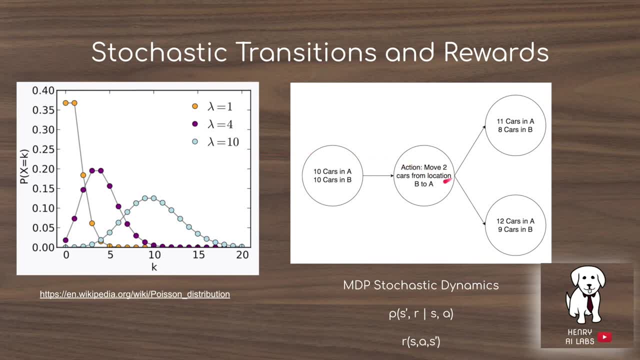 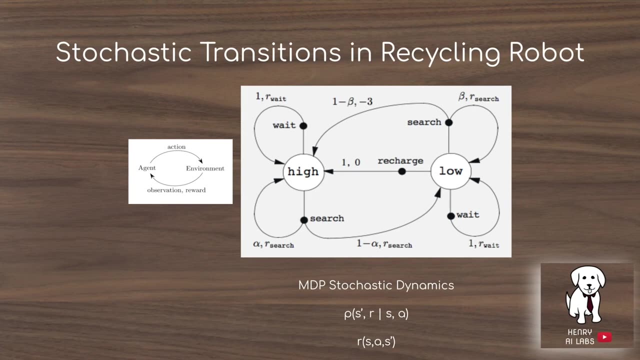 of probability distribution with respect to how the Markov decision process transitions from state to state given a certain action. Additionally, we have a stochastic reward variable now as well, because the demand is a random variable that isn't going to be the same every single time in every single state. So this is just contrasting to our recycling robot, in which the 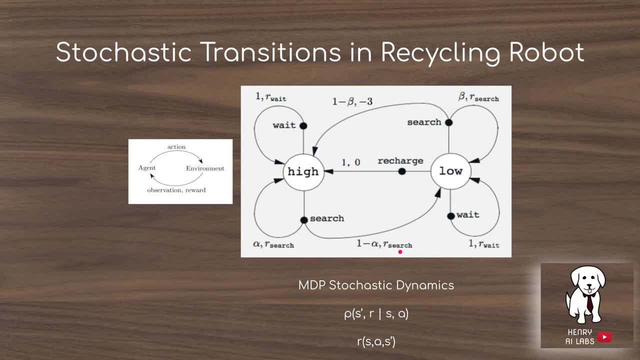 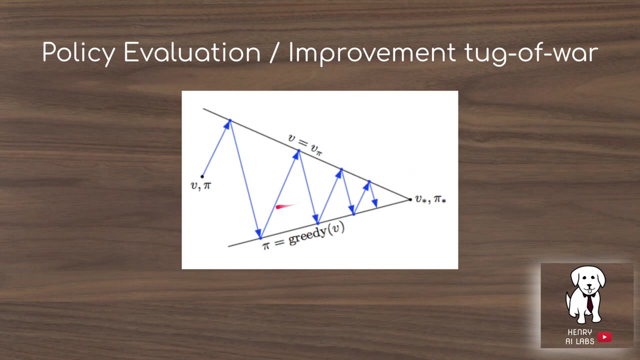 transitions are much more straightforward and the reward is deterministic. We have the same reward for every action in this toy problem. to motivate MVPs and understand this framework, We'll conclude discussing the generalized policy iteration algorithm with a couple of interesting characteristics about it. The first thing is this interesting tug of war between the evaluation and improvement. 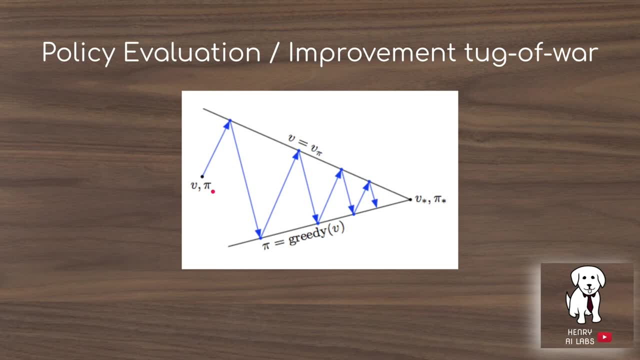 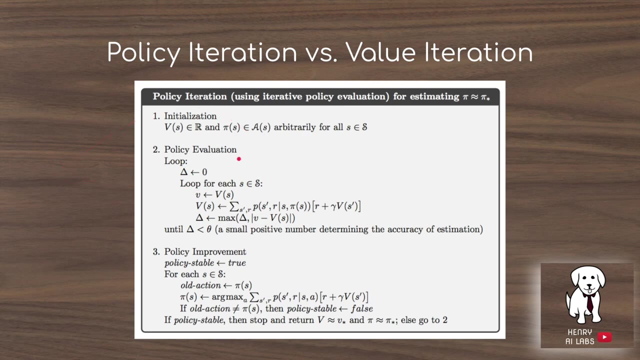 because every time we evaluate the policy and update our value functions then it makes the policy no longer greedy and then every time we make the policy greedy with respect to that value function, the value function estimate is no longer correct. Another interesting characteristic is our policy evaluation loop. So there is an interesting distinction in the book between: 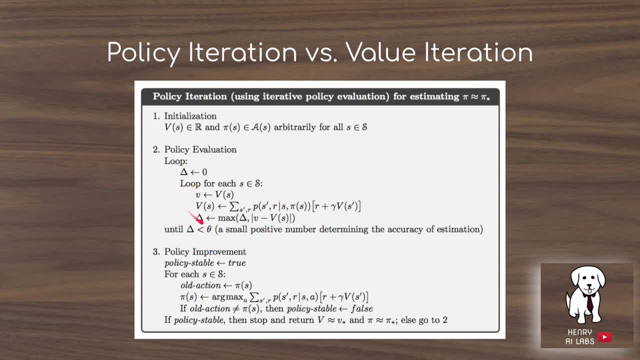 policy iteration, where we loop through several times until we hit this delta threshold and then exit out of the evaluation loop, compared to something called value iteration, where you only make one loop through this value update, despite whether it is completely converged to the correct state estimates. But the book gives you some convergence. 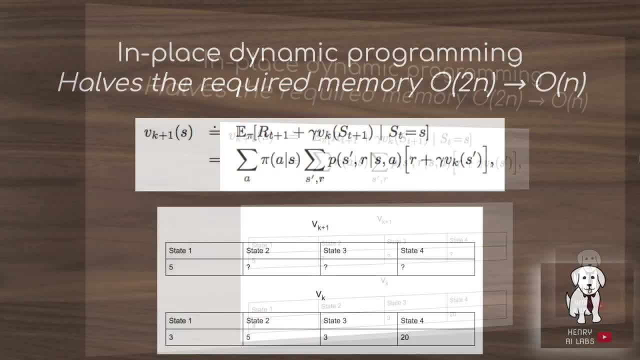 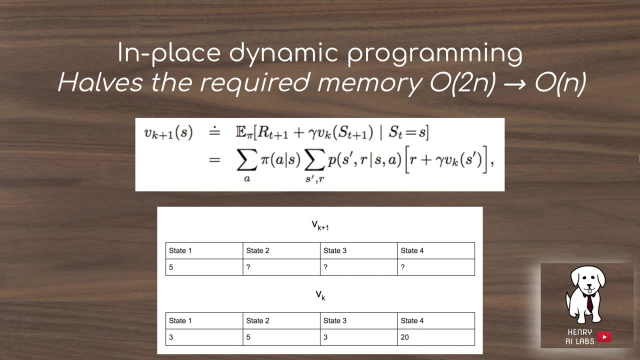 of why value iteration will still work in the GPI framework. Now we'll transition our presentation of the chapter from the generalized policy iteration algorithm to some characteristics of dynamic programming. So dynamic programming is a technique in computer science frequently used for things like genetic sequence alignment or like spell checking- Basically what you're doing. 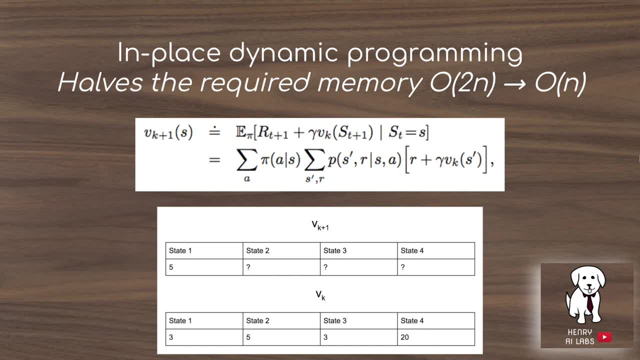 is you're bootstrapping the computation by using your estimate of v sub k plus one to estimate the state function with v sub k. So the in-place dynamic programming basically refers to this idea of not using a separate array that holds the previous value function estimates at time, step k. 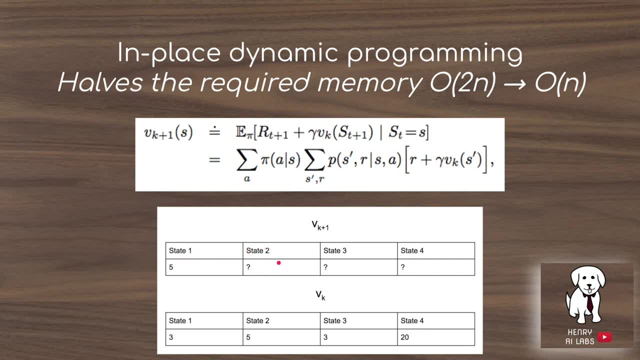 So what we would do, rather, is we update these state values in a single sweep with our Bellman equations and this might cause a little bit of noise in the updates, because you know, obviously as you update this state two is it might have like a higher magnitude of updating state three. You can imagine, 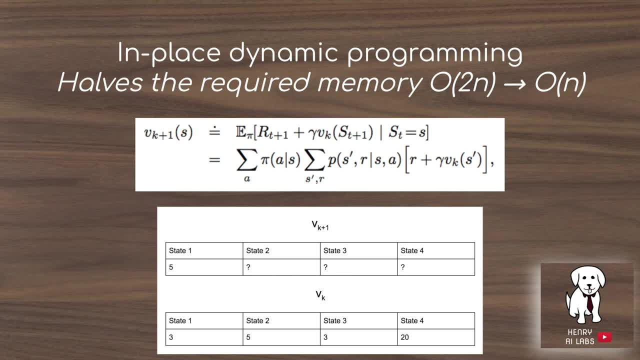 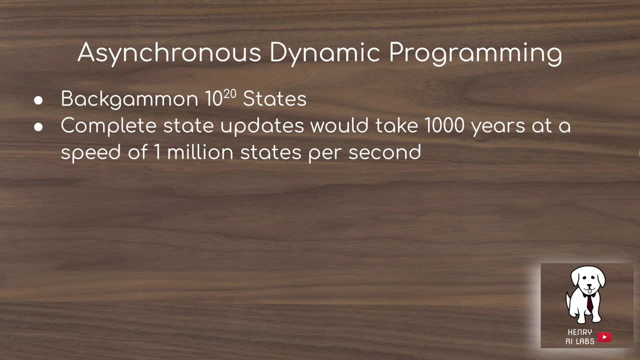 with the grid world example, how you traverse the grid and then how you update the values of every state is totally dependent on the previous updates. Another interesting extension to dynamic programming that makes it applicable to- you know, interesting reinforcement learning problems like chess and backgammon is this idea of asynchronous dynamic programming. So in backgammon we have 10 to the 20. 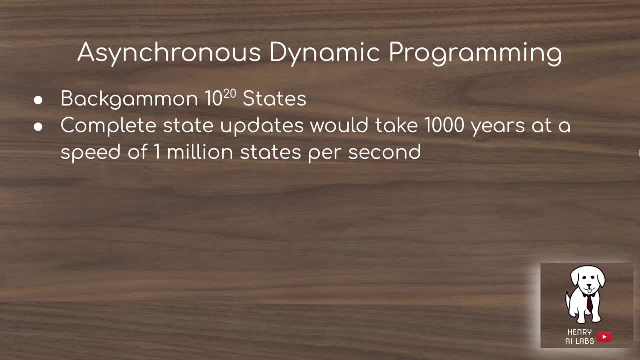 states. So the book motivates this problem by saying: if you were to do a complete state space sweep and update the value function estimates of all 10 to 20 states, that would take 1,000 years at a speed of 1 million state updates per second. So asynchronous programming, dynamic programming, 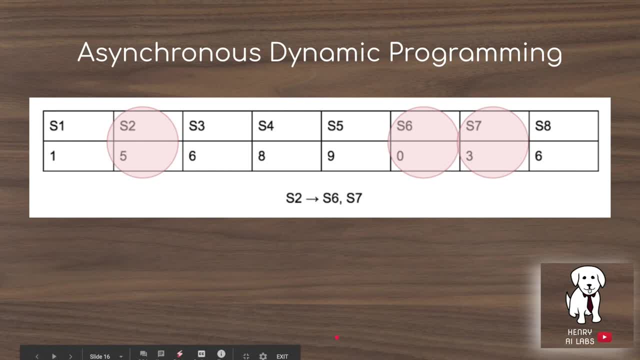 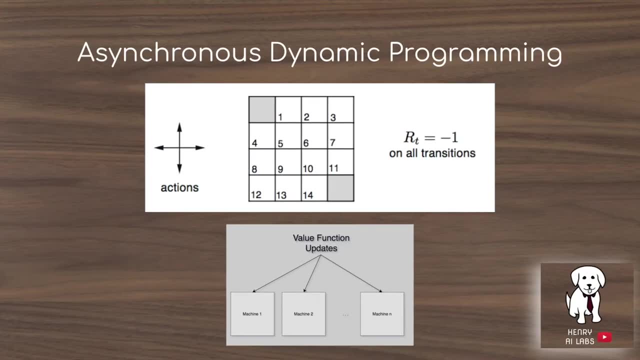 refers to this idea of updating the value estimates of a subset of states rather than the entire set of states in a policy evaluation iteration. So asynchronous dynamic programming can also be distributed across machines. So we can imagine sending, say, this top left half of the states in 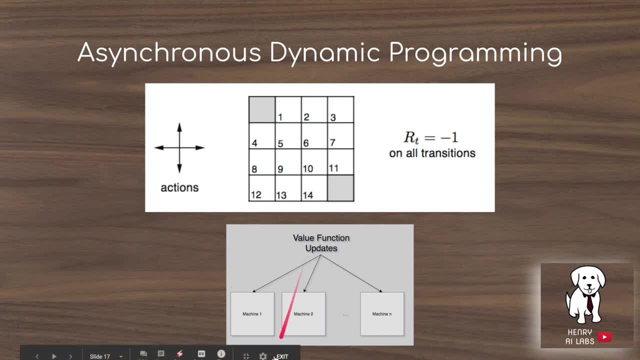 the value estimates to machine one, this top right half or quarter to machine two, and then you know distributing state spaces in this way and then you might have sort of a noisy value function update. but the book gives a more concrete example for how this will converge. The chapter also presents: 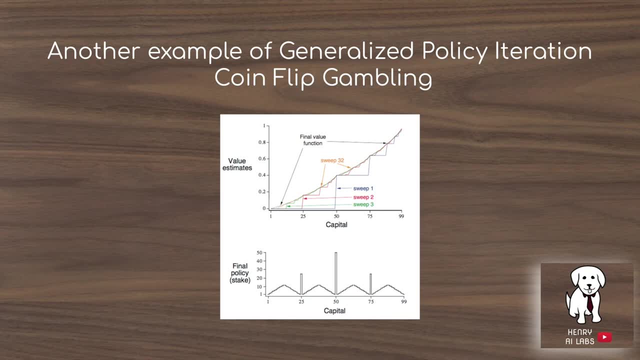 another example of generalized policy iterations. In this case you are betting your capital on a coin flip with a probability of p sub h equals 0.4, and then you're making this policy where you're deciding how much you want to bet given each amount of capital. So in this top chart you see how the 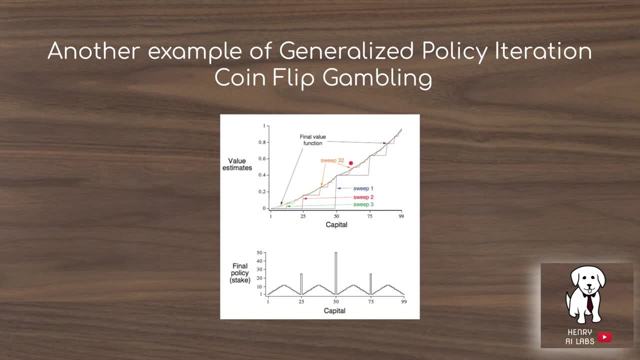 value estimate of the states are converging with respect to the iterative sweeps through the gpi algorithm. and then you see sort of an interesting policy where if you're at 50 you bet all of your money and if you're at like 51 you would just bet a little bit. see with the 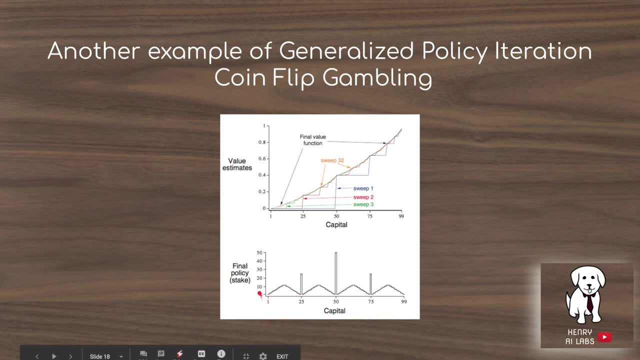 policy is the mapping from the capital state to the action being how much you bet on each coin flip. so it's an interesting little policy to see. and then this chart here is interesting to see, a visualization of the convergence of the gpi algorithm. thanks for watching this explanation. 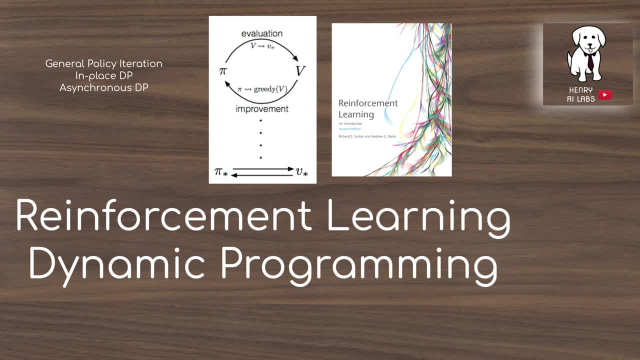 of dynamic programming, chapter 4 in the book, an introduction to reinforcement learning, by Richard Sutton and Andrew Bartaux. Hopefully from this video you took away the idea of generalized policy iteration and characteristics of dynamic programming, like in place memory tables and asynchronous updates. Please stay tuned for chapter 4..